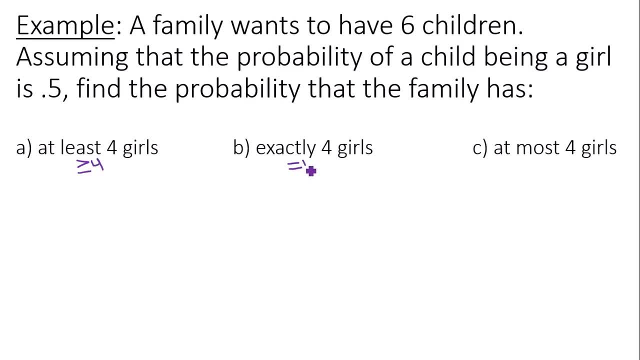 to four, exactly four girls, so that's equal to four, and at most four girls, so that would have to be less than or equal to four. Now it's clear that the behavior we're observing here is a child being a girl. so a success for a binomial experiment in this case is the child is a girl. 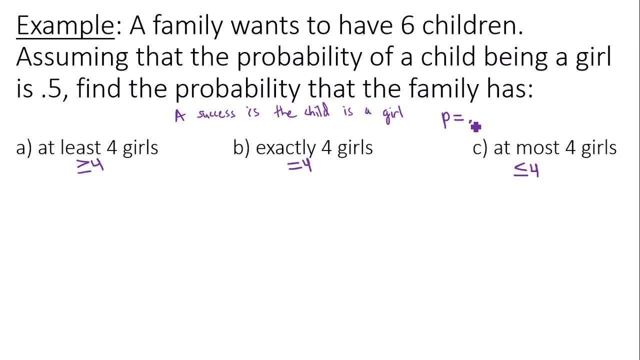 So that means that the probability of a success p is equal to 0.5.. Okay, so the Google Sheets input for each of these at least four girls. Well, first off, the number of trials or children being born is six. Probability of a success is 0.5. 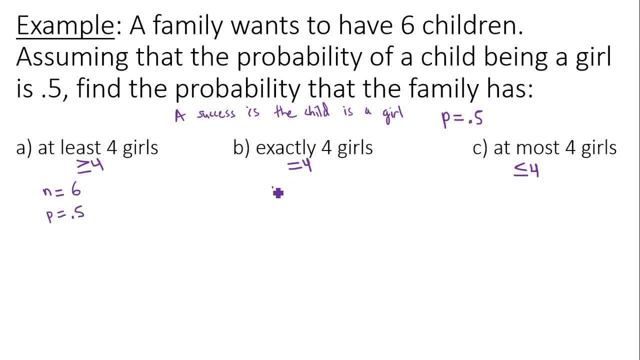 This stays the same for every single scenario. This never changes. What does vary slightly, though, would be your lower bound and upper bound- At least four girls, so that would be greater than or equal to four, So that's the probability of a success. 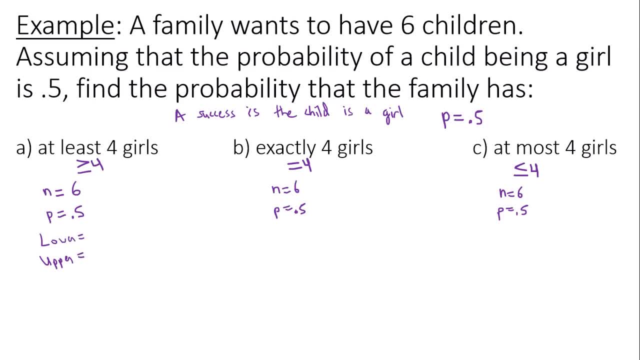 So if you're interested in at least four girls, this would mean four, five, all the way up through six. You can't have seven because you only have six children. You can never exceed the number of trials. So the lower bound is four, upper bound is six, Exactly four girls: the lower and upper 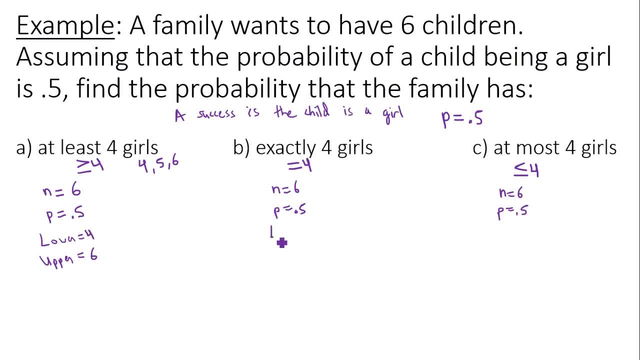 bound would be looking at just four. Lower bound is four, upper bound is six. So if you're interested in at least four girls, this would mean four, five all the way up through six. You can't have seven, just four. Lower bound, upper bound, is exactly the same. 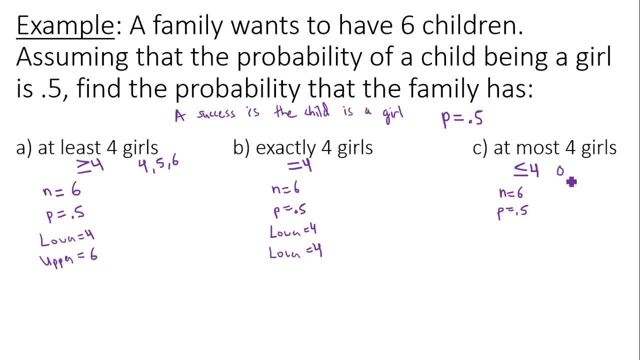 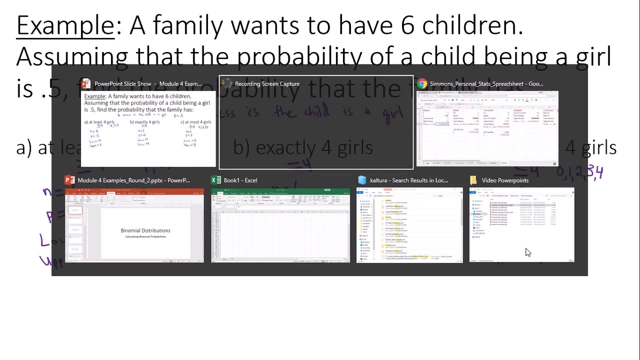 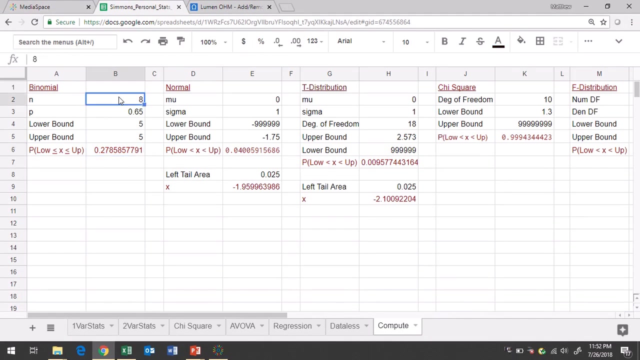 At most four girls. that means zero, one, two, three and even includes four. So the lower bound in this case is zero and your upper bound would be four. This is all the information you put into Google Sheets. If you're not there already, make sure you're in the Compute tab. 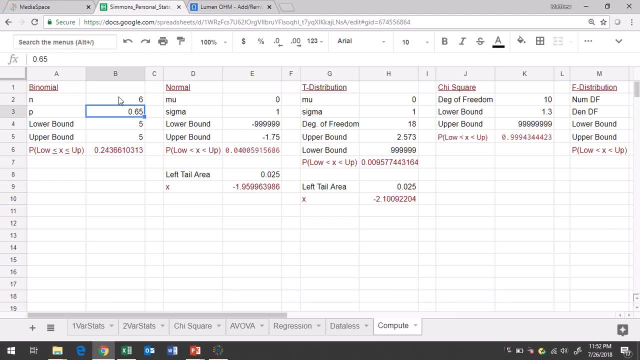 The number of trials would be 6, and then the probability of success is 0.5.. For my first part, my lower bound was 6 and upper bound was 4.. This gave me a probability of 0.3438, rounded to four decimal places.